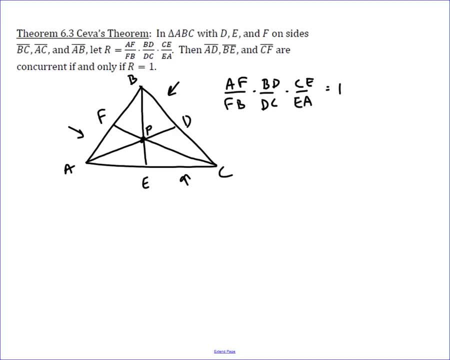 Or you could do it vice versa and it would work out as well, meaning, AE over EC equals CD over BV, which equals BF over FA. Either one of those works for this problem. But where you use this is in two ways. First off, you use it to prove…. 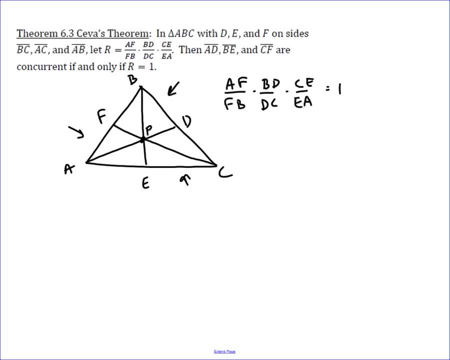 You use it to prove that three Chevins in a triangle are concurrent to each other, concurrent with each other, meaning they all meet at a single point. The other thing you can use it for is if they are concurrent and you know that, and then you know some other things about these side lengths, you can quickly find something else. 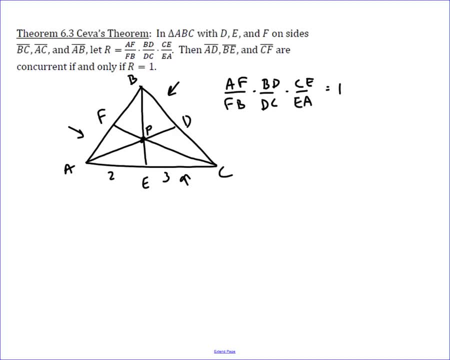 So, for instance, if you knew this was 2 and this was 3, and this was 4 and this was 5… Right, Well, if VD… VD over DC is 4 fifths, and EC over AE is 3 halves, and AF over FB, we don't know. 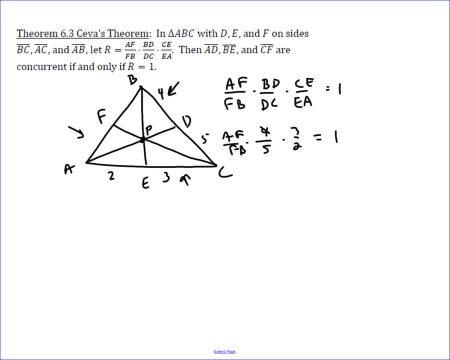 Well, you can find AF over FB very easily, in that it equals AF over FB times 6 fifths equals 1, multiplied by both sides, by 5 sixths and you find out that AF over FB equals 5 sixths. So a very nice…. 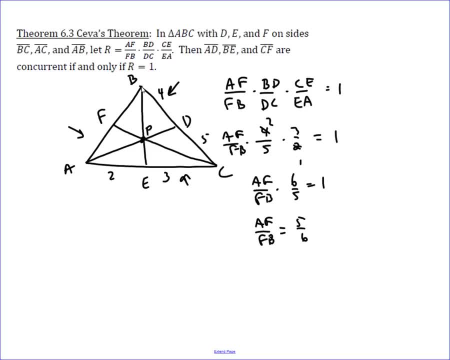 So a very nice application of this theorem. The proof of it uses one way to prove it. There's multiple ways to prove this And the one I want to talk about uses what we refer to as the ratio theorem and the area theorem, which says that in a triangle with a Chevin ABE, the area of triangle, ABP for some random point P on BE over area of CBP…. 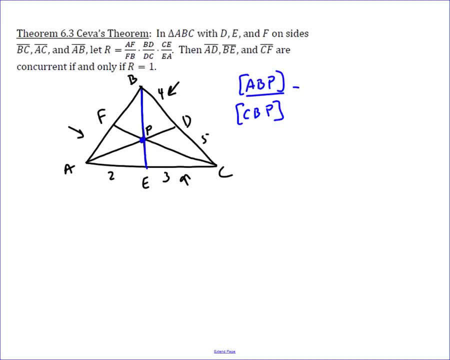 is just going to be equal to the value of the opposite sides: AE over EC. Okay so ABP over CBP, these two triangles right, where you're kind of using point P here – B in both of them. Well, if you look at the opposite sides, that's the ratio of the areas of those two triangles. 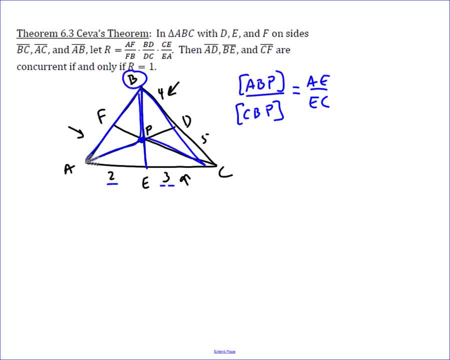 If we do that all the way around…. So, for instance, if we look at this triangle and this triangle… We could say the area of ABP – and actually, to make our life easier, we're going to do the area of APC over the area of ABP.